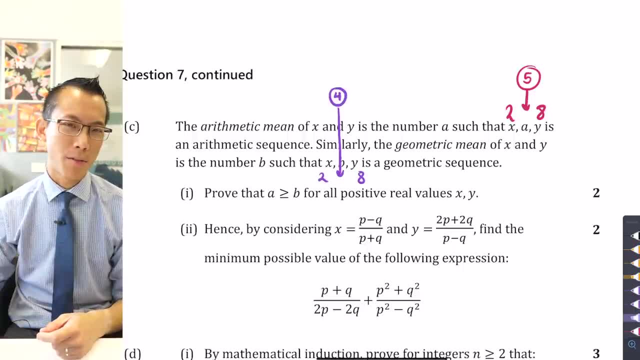 got a common ratio of 2.. I'm doubling every time. The next number would be 16,, 32, and so on. So in this case, the arithmetic mean, or the am for short, is 5, and the geometric mean, the gm for short, is 4.. Now what we're then? 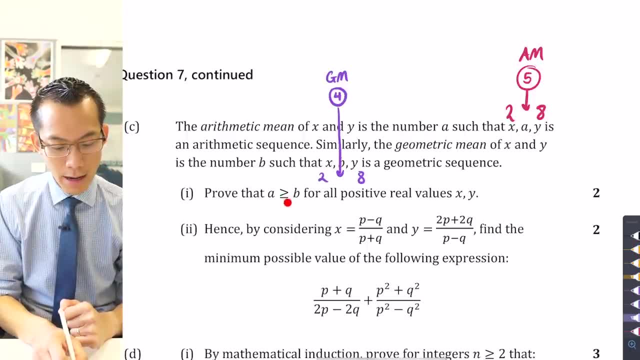 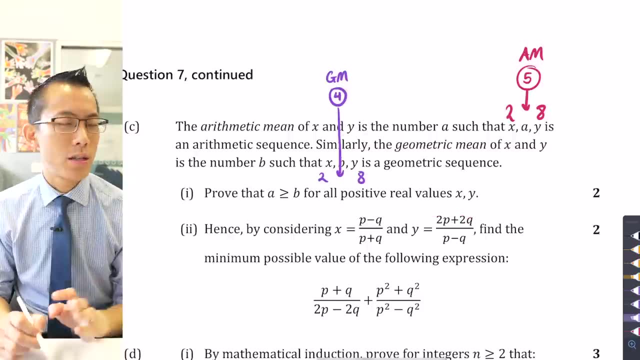 asked to prove in part 1 is prove that a is greater than or equal to b. in other words, that the am, the arithmetic mean, is bigger than the gm, the geometric mean for all positive real values, x and y. In other words, I didn't have to just choose 2 and 8. I could have 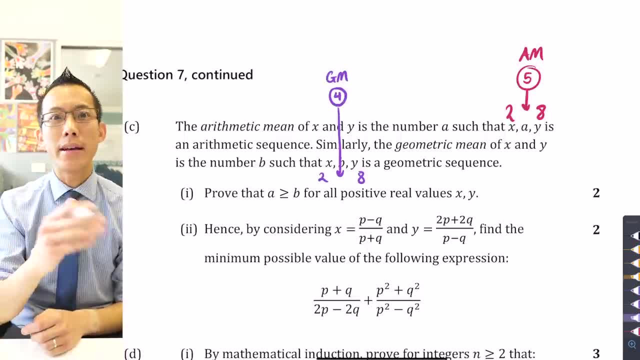 chosen any two numbers and the arithmetic mean will always be bigger than the geometric mean. How do I prove that? Well, you've really got to set this up to sort of make it easy for yourself, right? You can see, I just gave a numerical example so that I knew what I was going on with here. 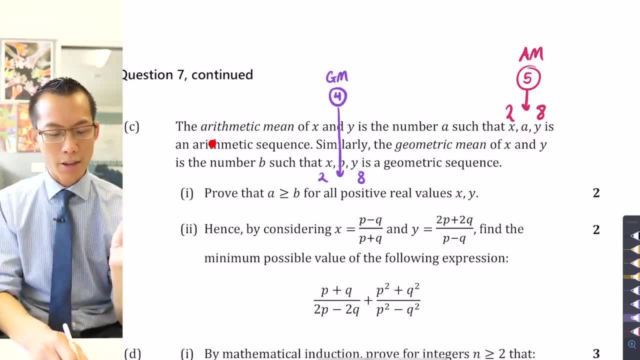 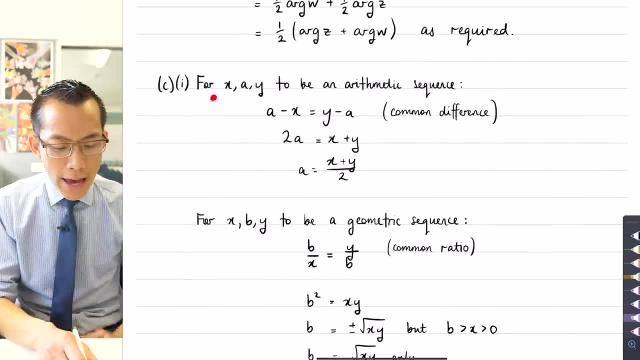 but in order to prove this particular result, I need to phrase the arithmetic mean and the geometric mean in such a way to make this easy for me to prove. So here's the way that I've done it: For x, a, y to be an arithmetic sequence, we know we've got a common difference, right? 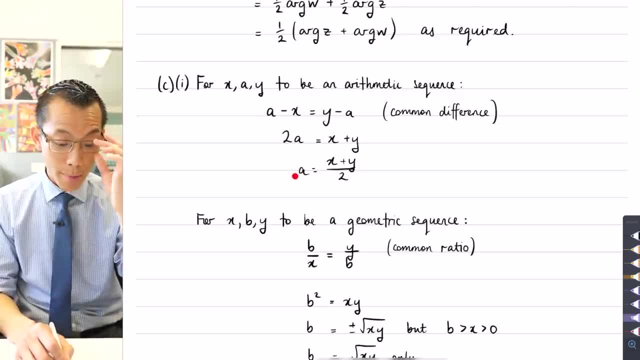 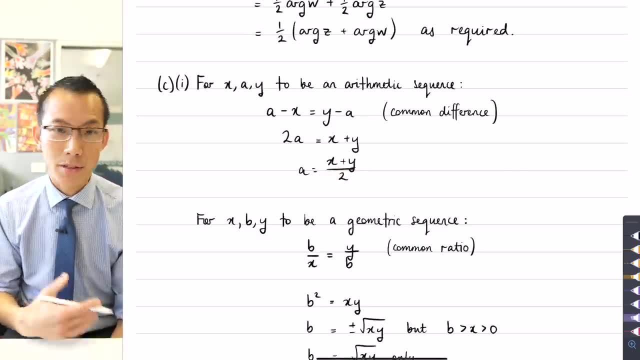 So this is the definition of that common difference. So you get the arithmetic mean being x plus y on 2.. Of course, you would think, is the midpoint formula, or this is the way that I work out the average of two numbers, because that's what we think of as the arithmetic mean. 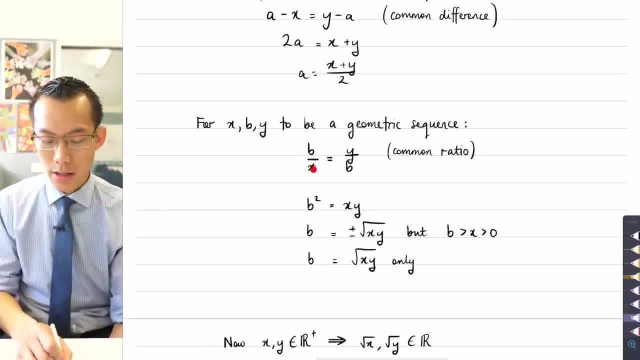 Here's the geometric sequence. You've got this common ratio happening between the pairs of terms, the consecutive pairs of terms, I should say. And so you've got b squared equals xy. and I don't want b squared, I want b right. So I've got plus or minus the square. 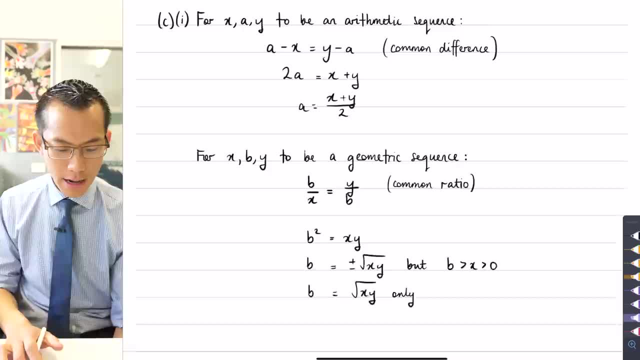 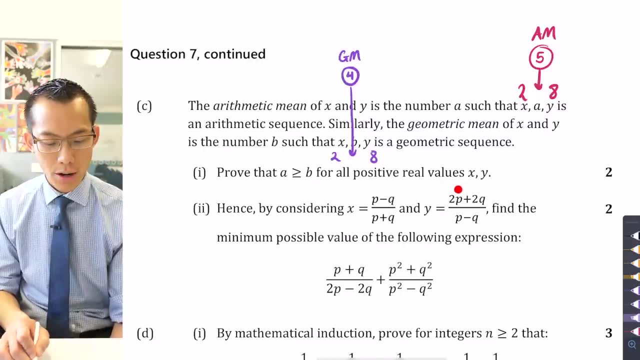 root of xy. I do note that if you have a look back at the original question, I've specified that x and y have to be positive real values. So in order to get a nice geometric sequence here, I want to specify for b being positive. 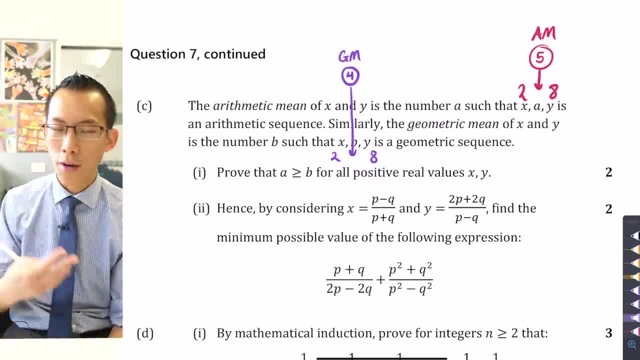 If b were negative? well, you know, a is positive, b is negative. of course a is bigger. But the whole point here is that no matter which geometric mean that I choose because I could have, I guess, put in negative 4 here and it would have still worked. just get a ratio. 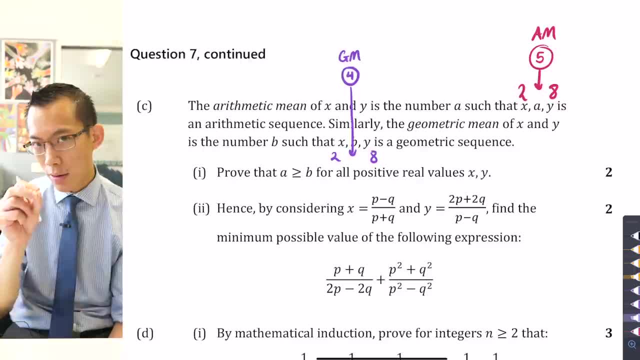 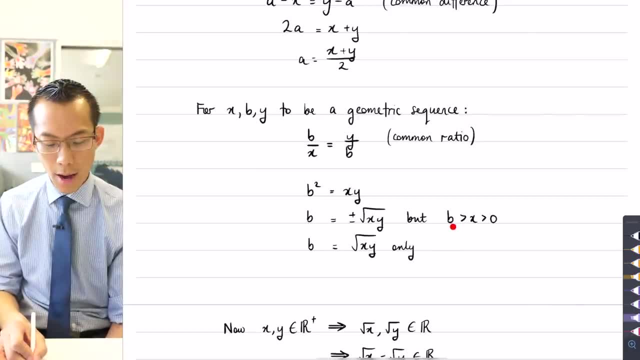 of negative 2, but that's a trivial result, right? So I'm thinking about the positive value that's in between them. Well, coming back to my solution, I'm specifying the positive value for b, the one that's bigger than x. It has to be bigger than x because between x and y, I'm going to get b being 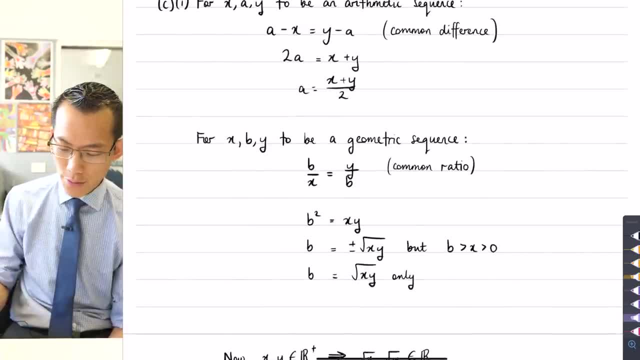 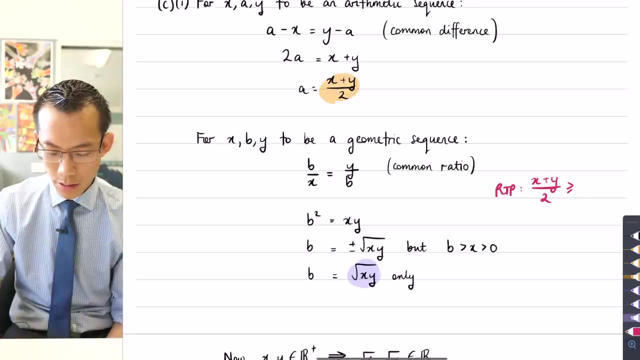 the square root of xy. So what I'm required to prove is that this result here, the am, is going to be bigger than this result here, the gm. So I guess I'm required to prove that x plus y on 2 is greater than or equal to the square root of xy. Now I'm pausing, right. 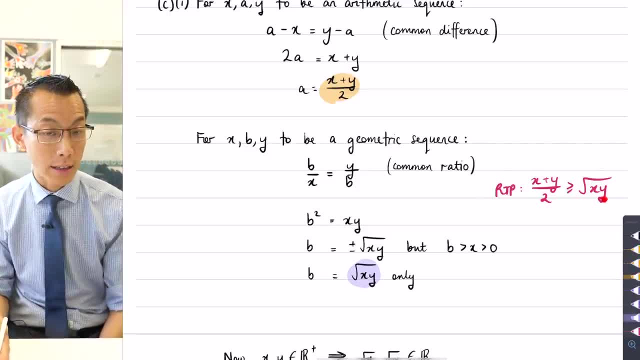 here for two reasons. Number one: it's always helpful to state very clearly what it is you're trying to prove before you start to prove it And whilst most questions, as you can see in this paper and in the HSC and any other exam you're going to have when you're proving- 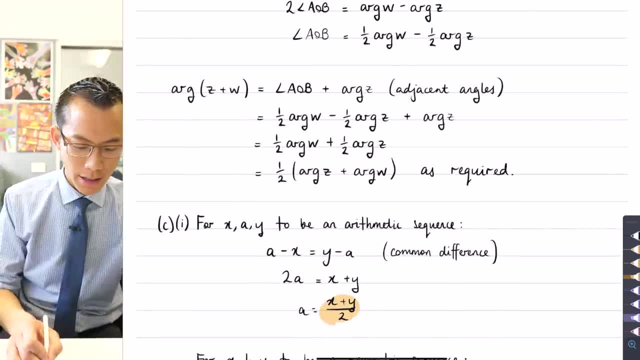 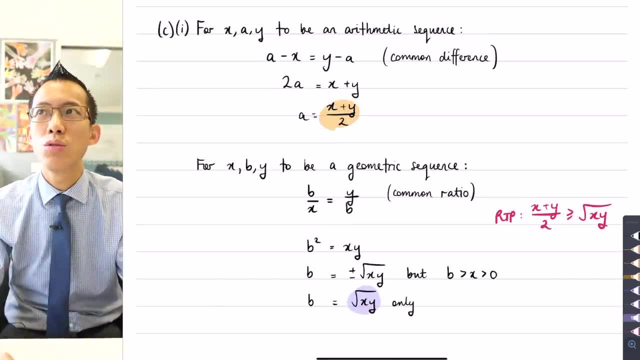 something they tell you, exactly what they want you to prove. Like. just look at the previous example. Like: here is the actual equation. I want you to prove this. This question made it a little bit more challenging by requiring you to articulate yourself what you had to. 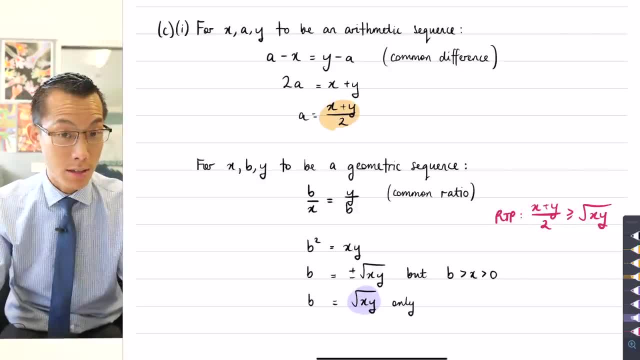 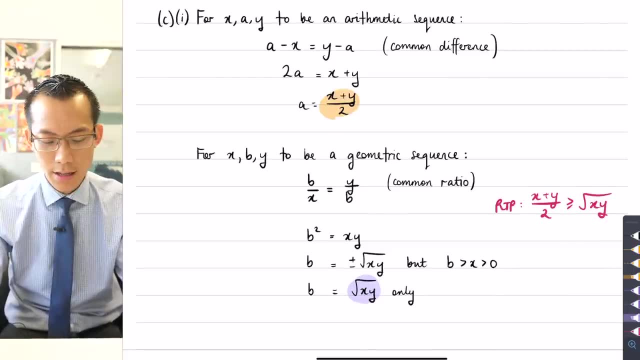 prove and then work out the path there on your own, which is an additional level of complexity. So there's the first thing- Sophistication, I should say. That's the first thing I want to state. The second thing is: one of the things we're consistently doing is recognising 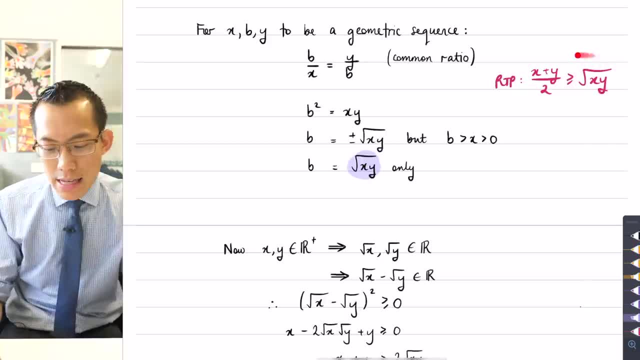 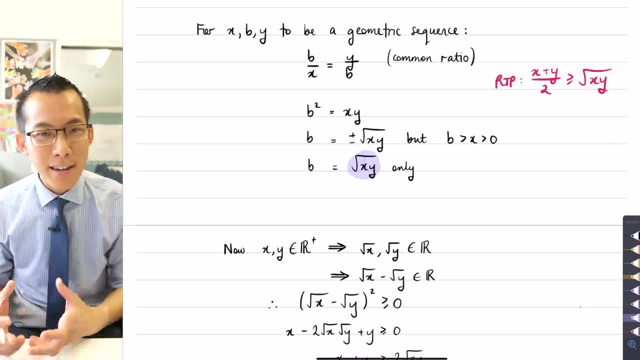 oh, I want to prove something. And then the first thing that you write is that thing you're trying to prove. And then you go ahead and you do some valid algebraic manipulation, but you don't get anything meaningful because you started off assuming the thing you were. 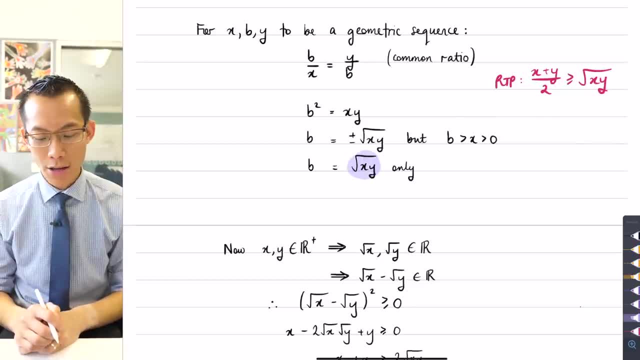 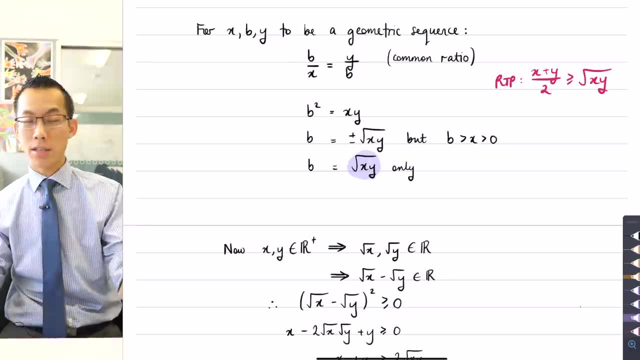 trying to prove, And that is always problematic. You can apply legitimate logical, logical, mathematical operations to something false and then arrive at something true. That doesn't mean the premise was true, but you can do things very simple, Like say, for instance: 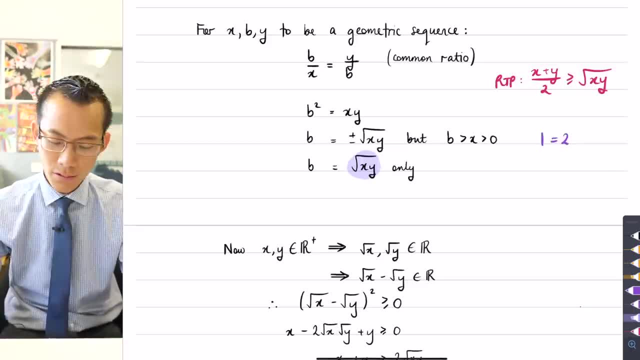 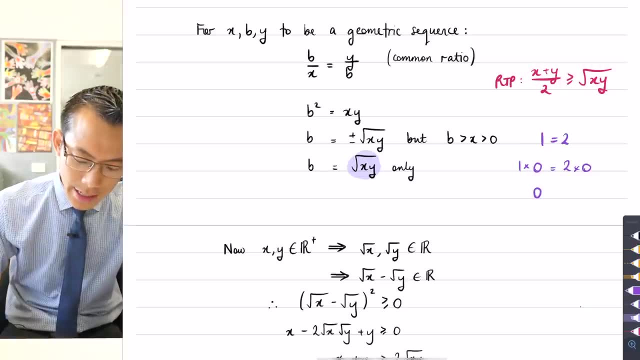 if I start off assuming that one equals two, which is not true, if I multiply both sides of this equation by the same number, which is a valid mathematical operation, I end at a statement that is true, but it does not follow that the statement that I began with. 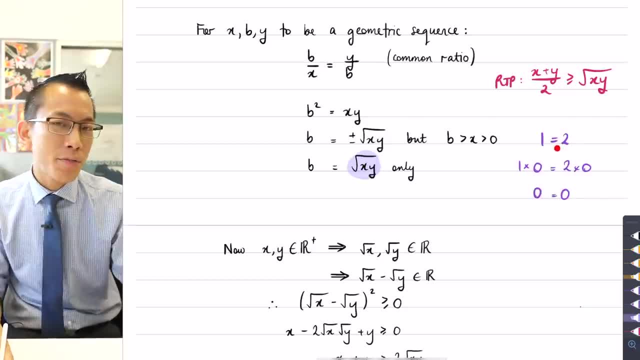 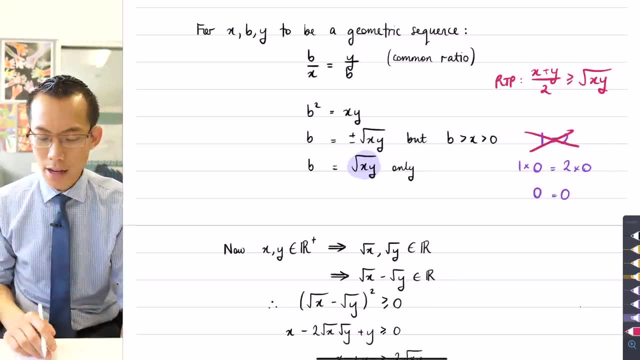 was true. even if what I ended with was true, This is a fallacy. So you cannot begin to prove something by assuming what you are trying to prove. It's a constant and easy mistake to make. So even if you say, yeah, this is where I'm headed, please do not start. 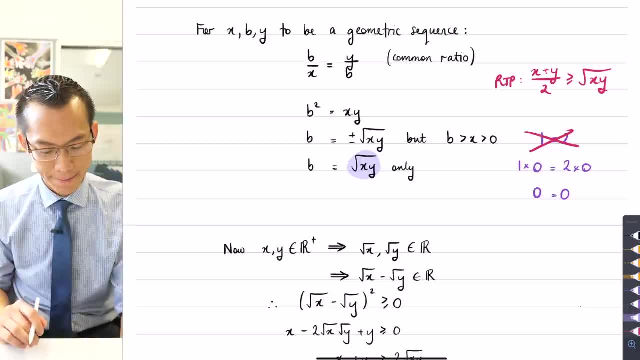 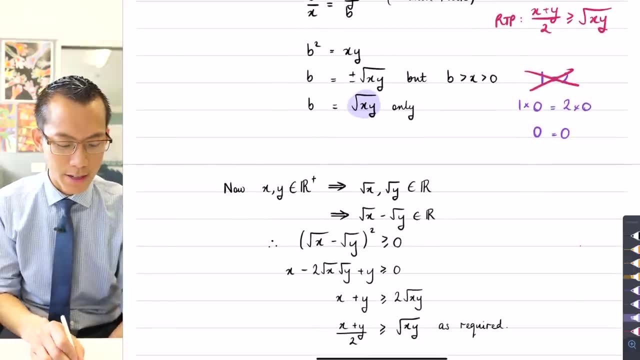 your working from there. Your working needs to end there, not start there. So, as I mentioned before, it's often, you know, this proof becomes easy if you know how to set it up. So what I've done is I've said x and y, they're going to be positive. 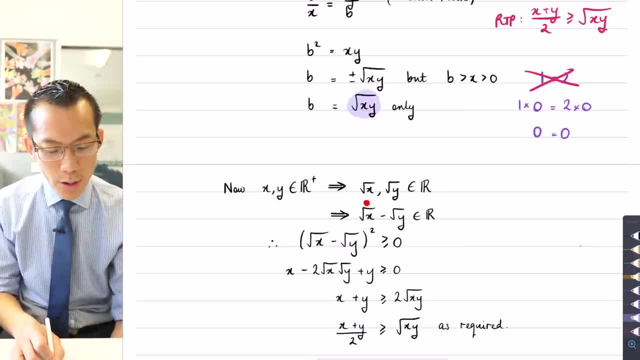 real numbers. That was given to me in the question, And that means the square root of x and the square root of y will also be real numbers. I wouldn't be able to do that. I wouldn't be able to do that. I wouldn't be able to. 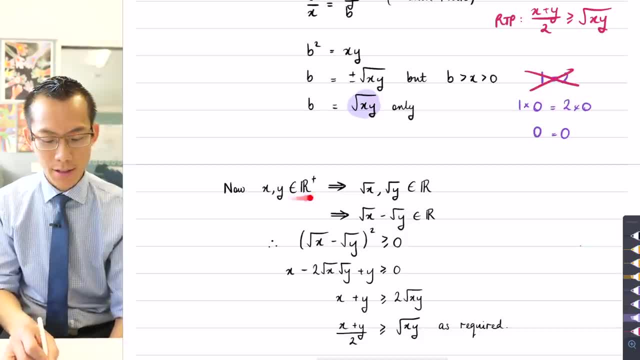 say that all the time. If x or y were negative, for instance, then the square root of x or the square root of y might be imaginary. but I've already been restricted within positive real numbers, So I can say the square roots are also real numbers If you've got two numbers. 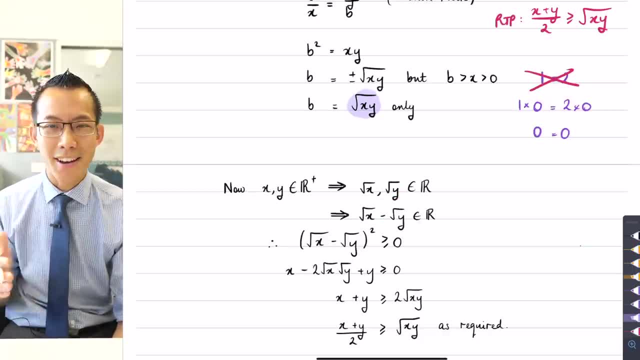 that are both real and you take the difference between them, there's no way for an imaginary component to sneak in. So therefore the difference between two real numbers is also a real number. So there we go: The square root of x minus the square root of y is real, And that leads 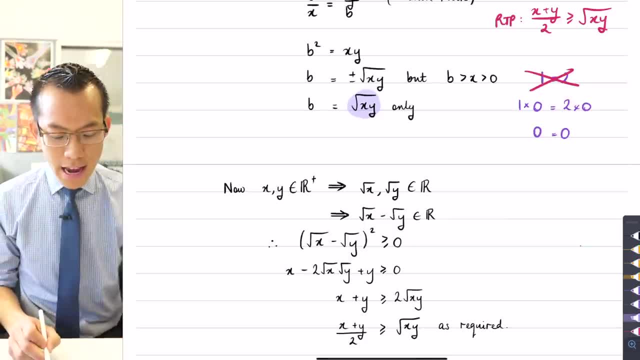 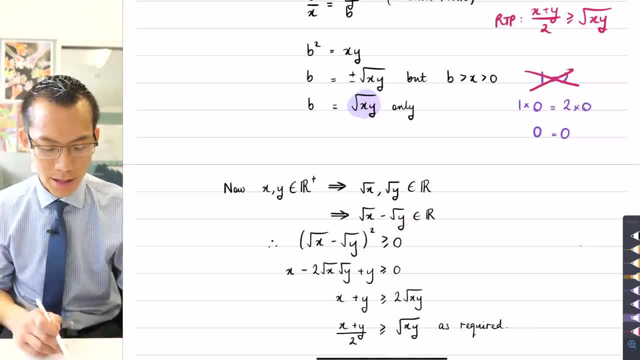 me to finally. Now I've got an inequality I can manipulate. If you square a real number, then the smallest it can be is zero, because you know the real number that would give you. that is zero itself. If you wanted something negative, you would need to have an imaginary number up here and 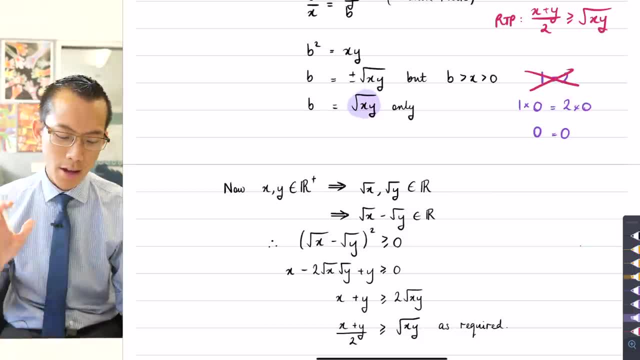 square that, But I don't. I just went to great pains to prove that the square root of x minus the square root of y is real. So therefore, when you square a real number, it has to be greater than or equal to zero. So many students just said this without providing evidence. 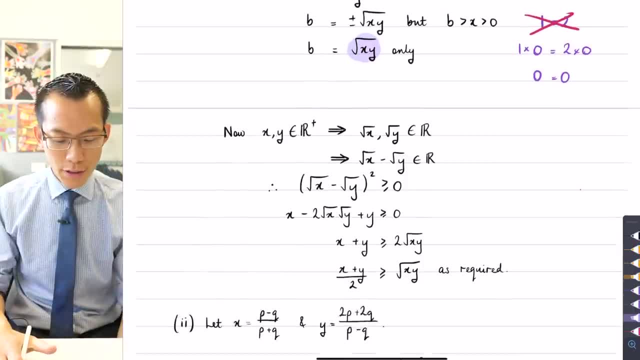 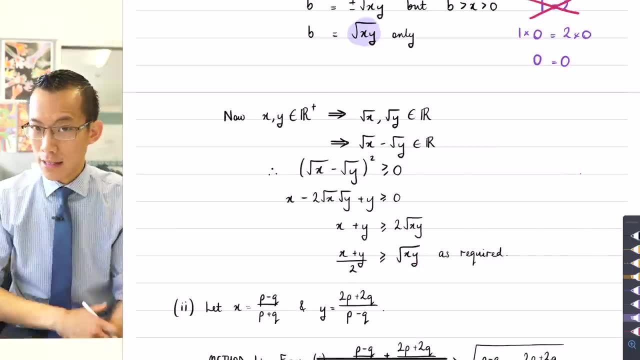 for why squaring? So I can't just say that it should give you greater than or equal to zero? and then all I have to do here is some fairly straightforward algebra. I expand out, I just get this over here on the right hand side and I divide by two to get the am on one side and the gm on. 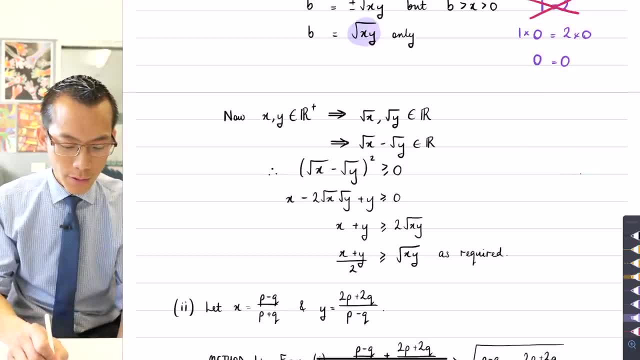 the other. So that's what I would advise. A lot of students sort of caught themselves in twists because, instead of dealing with the square root of x and the square root of y, they just dealt with something like, say, x minus y, all squared. Now that's not wrong. 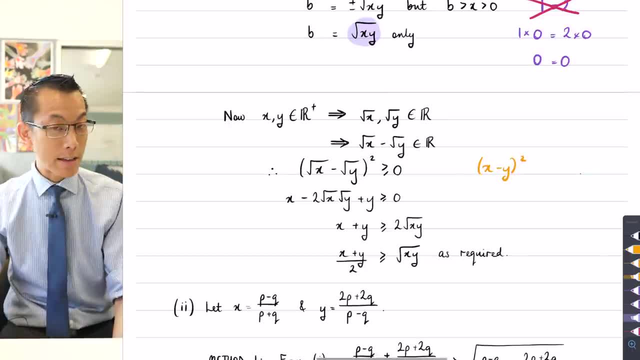 x minus y, all squared. You might still say that x minus y, all squared. That's not wrong. You might still say x minus y, all squared. You might still say x minus y, all squared, Now, that's not wrong. You might still say x minus y, all squared. You might still say x minus. 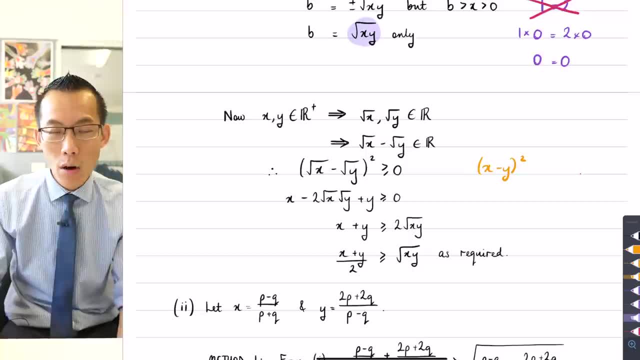 say: well, x is real, y is real, x minus y is real. so therefore, when you square it, you get something greater than or equal to 0.. So you ended up with something like this: Now you can get to the result that you need from here, but there's two. 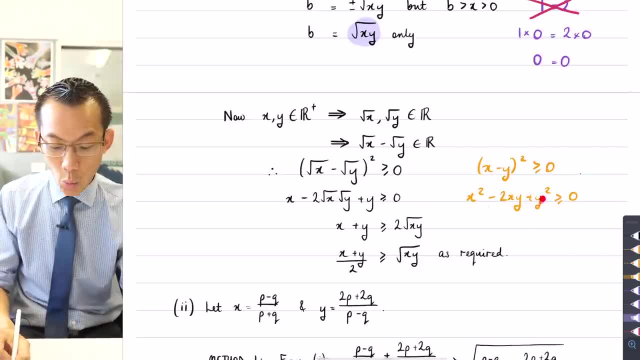 reasons why it's more complicated. Number one: you've got to deal with these squares in here. that's tricky. and then, number two, you actually end up having to take square roots of both sides in order to turn this xy into a square root of xy. 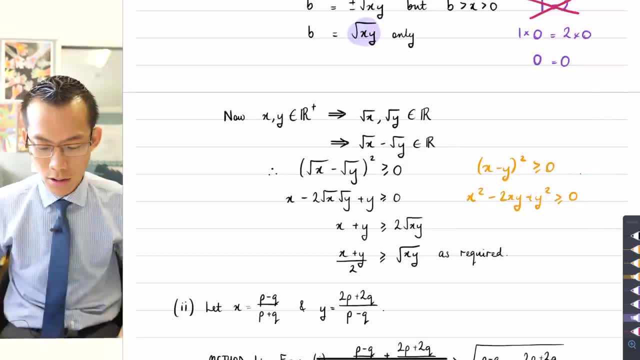 and you have to be quite cautious when you're taking square roots on two sides of an equation or an inequality. You've got to be careful with positiveness, with parity- that's oddness and evenness. you've got to be careful with sign, which is 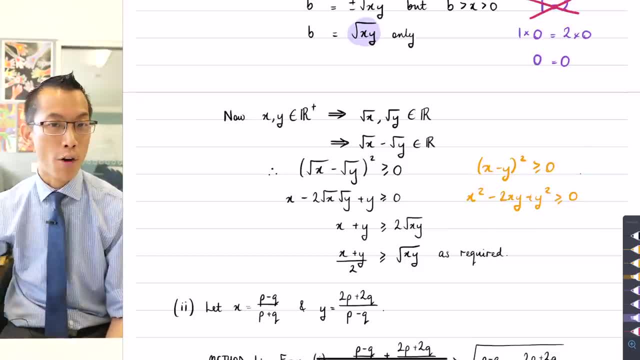 whether it's positive or negative, and a lot of people just took the square root of both sides of an inequality without making any statements as to why you could take square roots and you preserve the direction of the inequality. So great care needs to be taken, which is what I was doing up here. I started with the 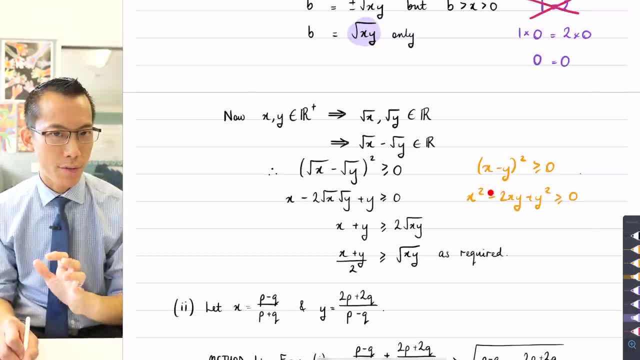 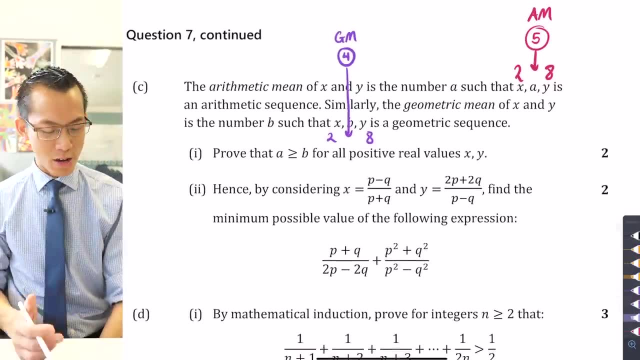 square roots of x and y. but if you do this path, you just have to take care of the positives and negatives later. Okay, so that was part one. What do we then do with this am-gm inequality? Well, it says: hence, which means you had to use that result by considering: x equals this and. 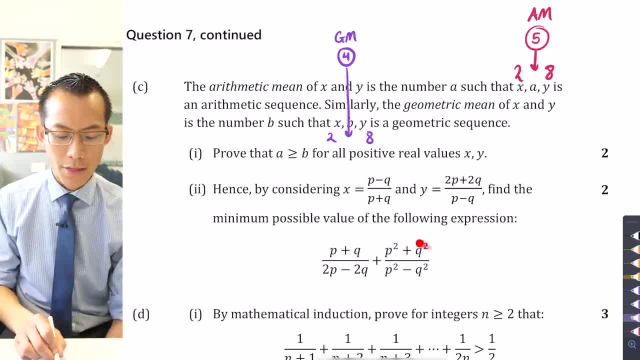 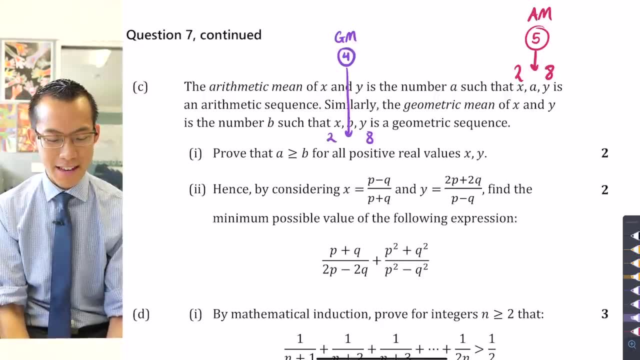 y equals this: find the minimum possible value of this gross, messy looking expression. How do we go about doing this? Well, please note that the question does say hence. so you're going to have to use the am-gm inequality somehow, and I know that's a bit counterintuitive because most people who see this phrase 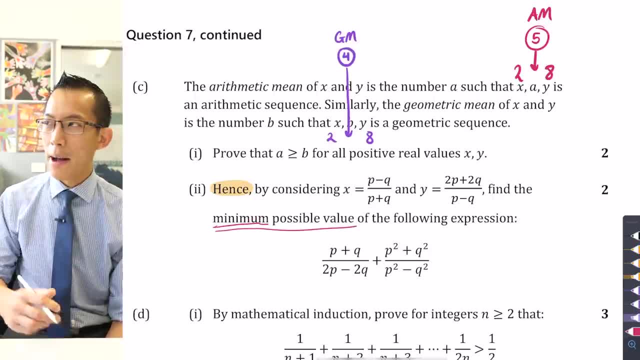 minimum, or indeed minimum possible value their brain, their advanced and extension. one brain says, aha, calculus, better differentiate and find a stationary point somewhere. Okay, now there's two reasons why you know that should not be the path that you take. Reason number one: they told you use the. 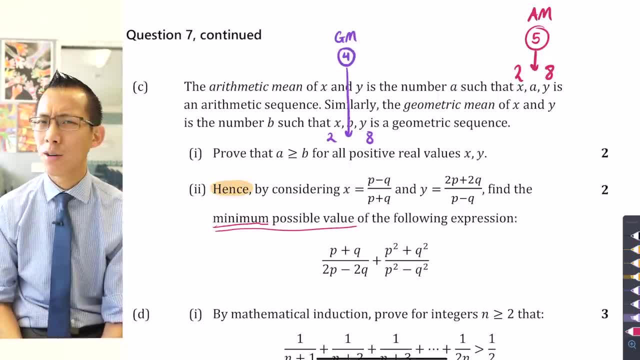 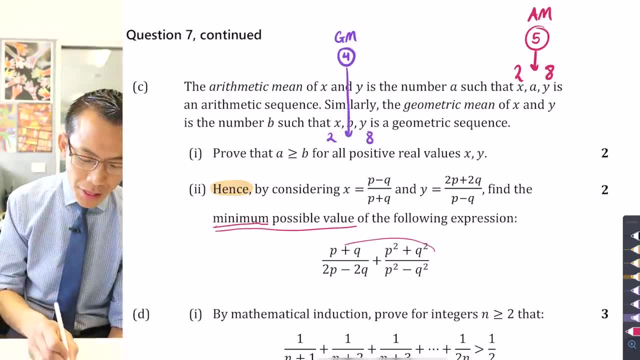 am-gm inequality, which we just used earlier. How do you use an inequality to find a minimum possible value? Well, I'll get to that in a second. I mean, the second thing is how you know not to differentiate This expression that you're dealing with here. let's highlight it rather than. 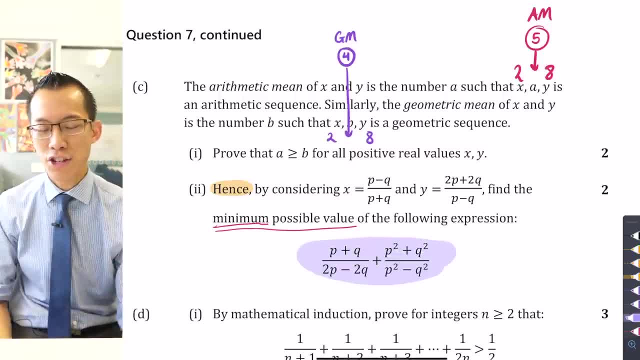 drawing a messy oval around it. This expression you need to differentiate. it depends on two variables: P and Q. It's a multi variable expression. If you were then to differentiate, what would you differentiate with respect to? Would it be P or would it be Q? If you did it with respect to P, you'd have to treat Q as. 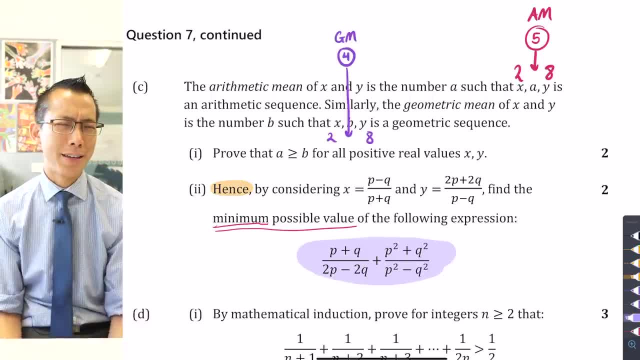 constant or vice versa. We haven't handled expressions like that in the course. You don't, unless you get to university and do something called a partial differential equation, which means you can take a multi variable equation or expression like this, which has P's and Q's, or 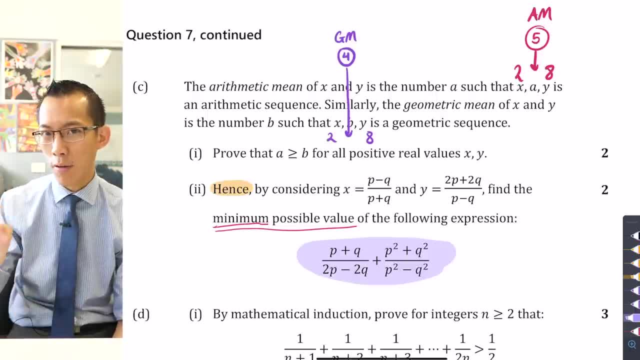 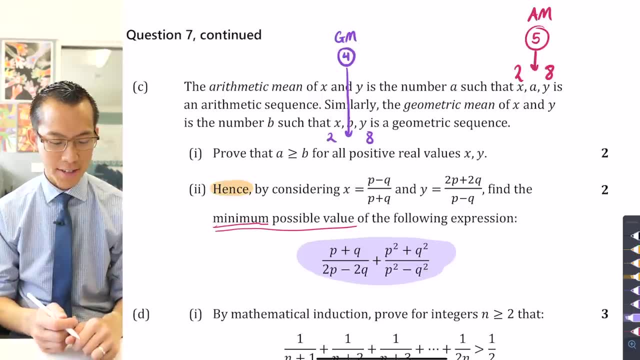 theta's and R's and you can differentiate with respect to just one of the variables. But no dice, here you've got a P and a Q. you're going to deal with both of them. So differentiation calculus are not the answer. What do we do instead? 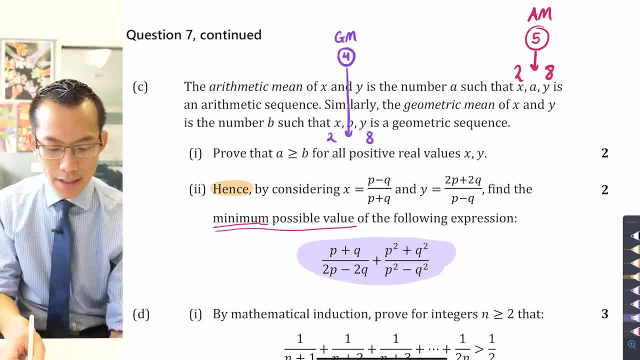 Well, the question again gives you massive clues. You've got this X and Y up here from the original question and then the question suggests: hey, let's do a differential equation. So I'm going to loop through the solution and then let X equal this, Let Y equal that, and then see what happens. So I'm going to show. 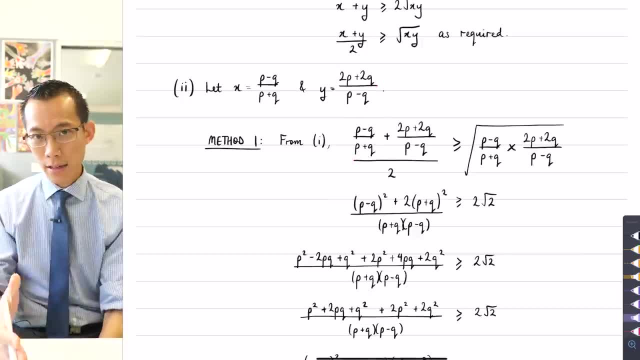 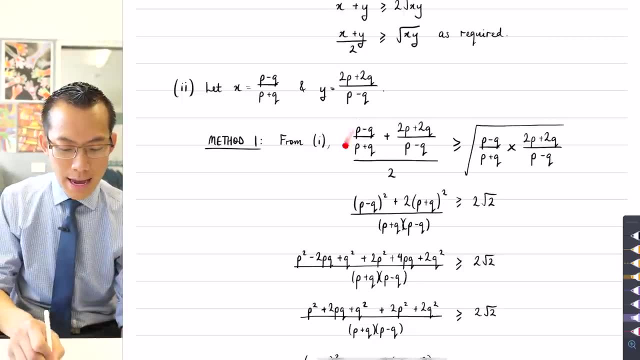 you how my solution unfolds. If X and Y take on these values, then what I can do is I can put that X and that Y directly into the AM GM inequality that I proved in part 1.. So here's the AM right. can you recognise that? Here's the X plus Y. 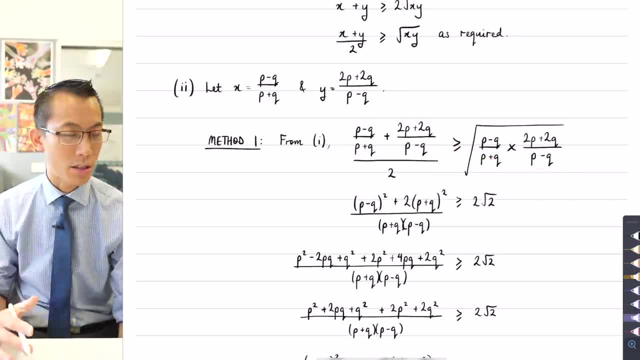 and then here's the square root of x, y. that's it, and i've just done a straight substitution. you can see on the right hand side you've got a whole bunch of cancelling. that happens. you've got this cancels with this. you've got- just be careful here- the p. 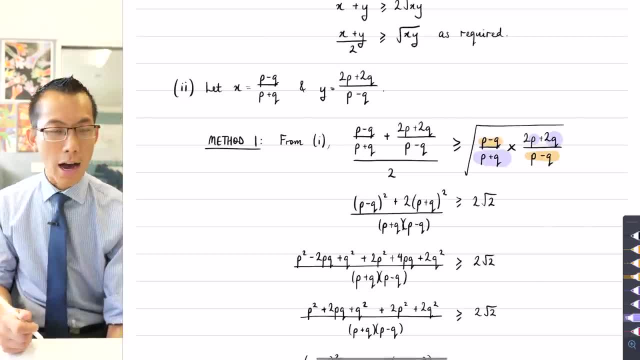 plus q cancels with the p plus q that is in that top numerator. after you've taken out that factor of two and the two that's left up here. once you factorize it out, that's what's left underneath the square root here: square root of two. 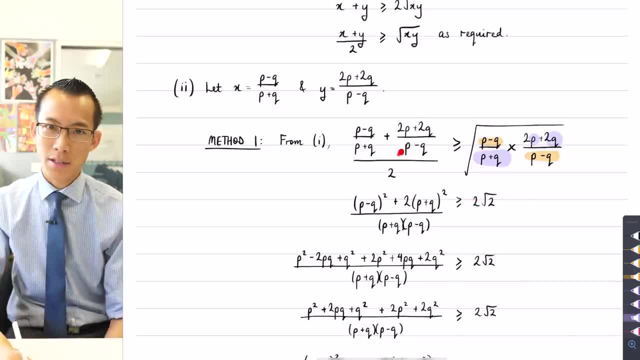 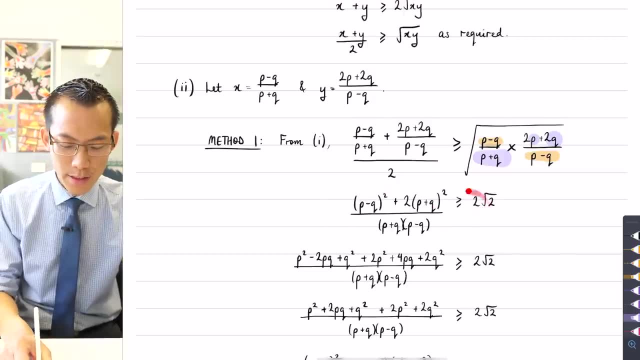 just for convenience, because i've got this fractions on fractions business over here on the left hand side. i've multiplied both sides of the equality by two, so that's how you get two root two over here. and then, lastly, in this first line of working, i've said whoa, what's going on? 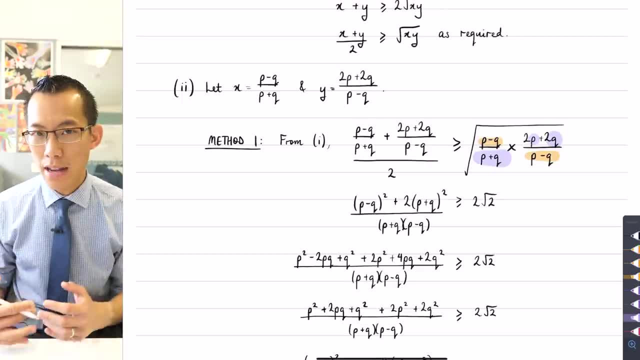 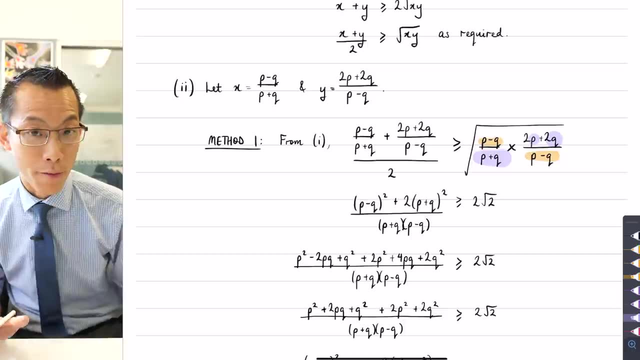 here with these two fractions, my most instinctive thing is to combine them into one by getting common denominators. now, it is worth noting that i'm not going to leave them as one fraction, because if you think about the result we're trying to prove or the expression we're trying to understand, 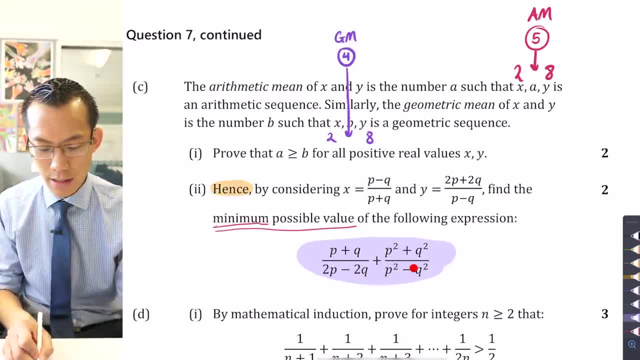 it's got two fractions, yeah, so i don't want to just keep these as a single fraction, these terms. when i add them up, however, i also notice that the denominators are rather different. you've got a p squared minus q squared here, which i can factorize into p minus q p. 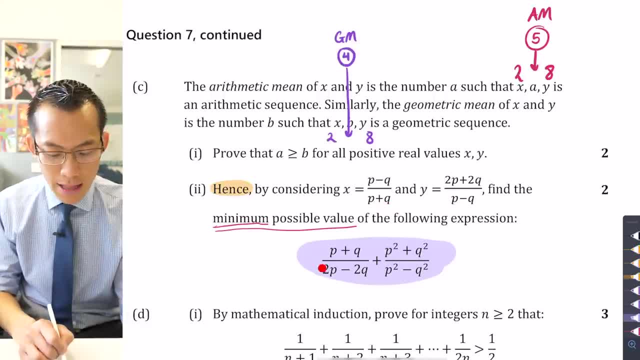 plus q. so you're like, oh, that's going to come from this common denominator, and then you've got 2p minus 2q, which- um, it might be helpful if i wrote this down: these- this also you can see- comes from this denominator over here. it's just. 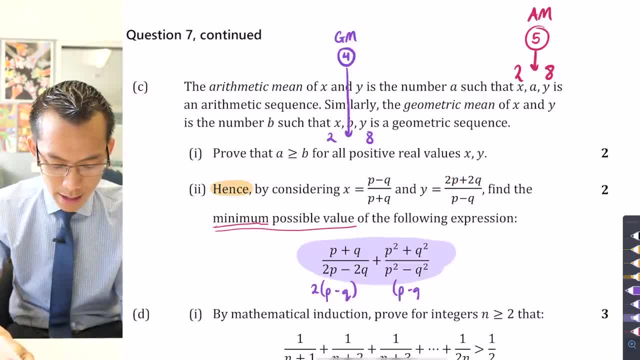 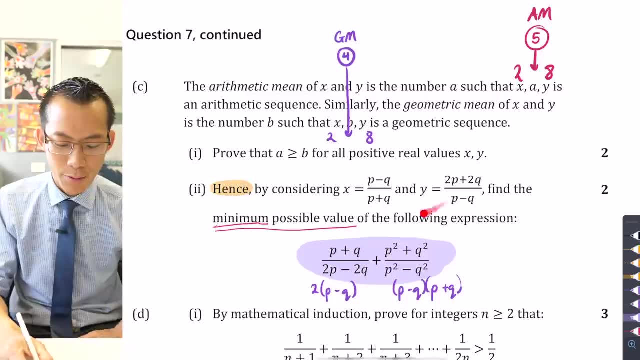 somehow looking backwards over there, so you can see that i'm going to eventually separate out again into two separate fractions. it's just not these fractions that i've started with here. i definitely don't want a p plus q over here. i'm going to have to do some. 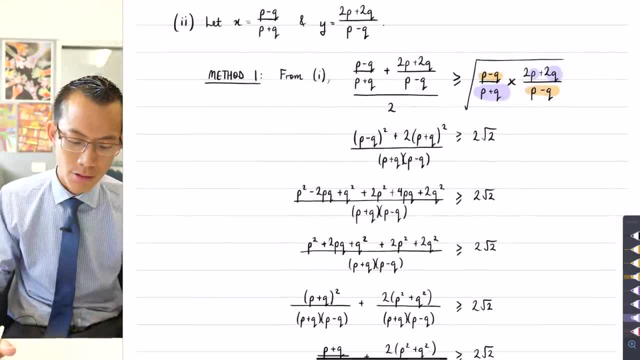 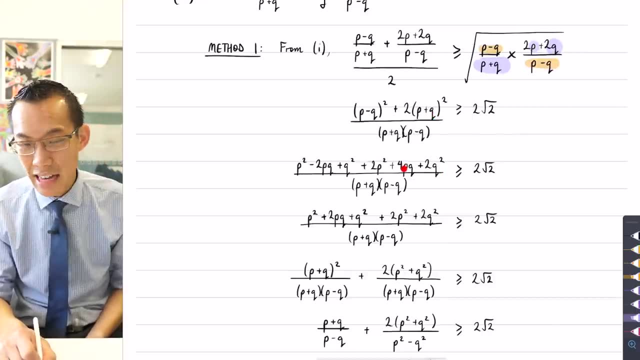 more um work with that. okay. so coming back to my solution, here you can see what i've done is i have got the common denominator. i've got this mess up the top here, but i've just expanded. that's why it looks so messy. i've got some like terms, but i haven't just sort of put them together. 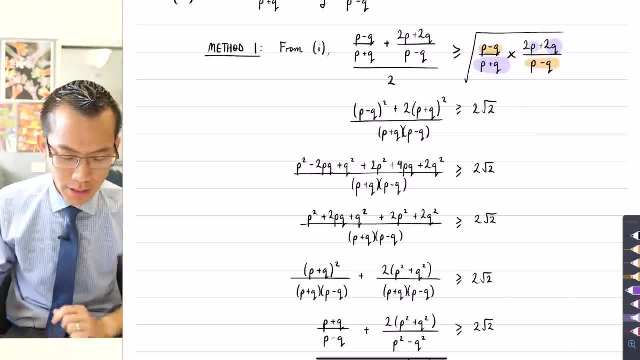 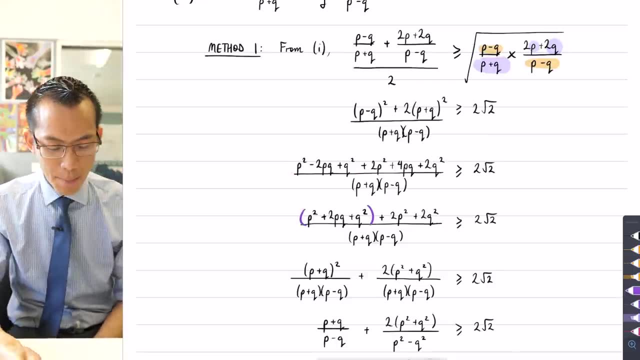 uh, what's the word i'm looking for, indiscriminately right? um, for example, you can see here what i've got from this: uh, not that one there wrong line, what i've got here, the p squared plus 2pq plus q squared. you might say to me, you know how come you didn't. 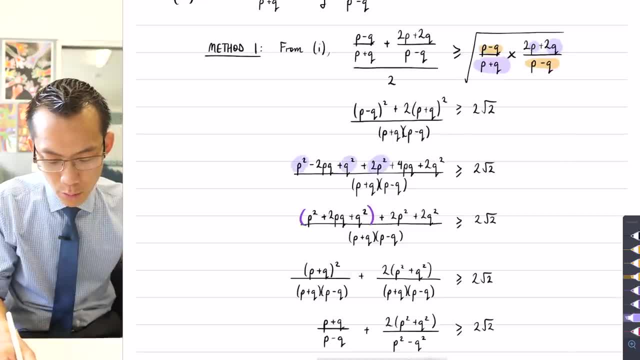 uh, combine the like terms p squared, q squared with 2p squared, 2q squared. a lot of students did that and said 3p squared plus 3q squared. not not an unusual thing to do, but also not a helpful thing to do, because you can't then factorize that. 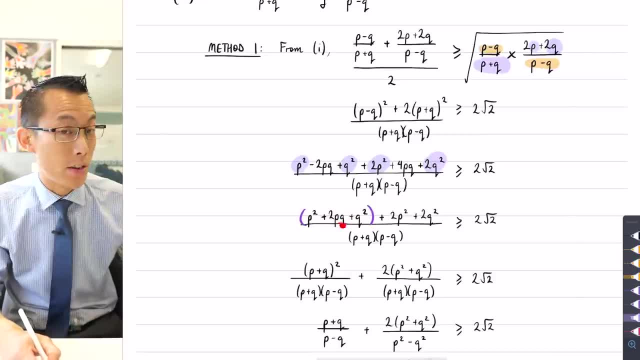 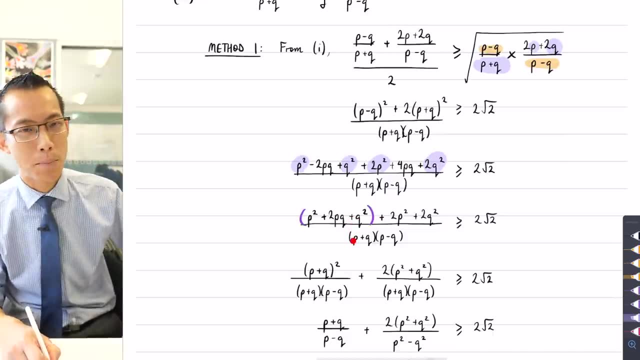 easily, whereas what i've got over here on the left, that's a perfect square. it's p plus q or squared. why would i want p plus q all squared? and the answer is it's going to cancel with one of the p plus q's down here. 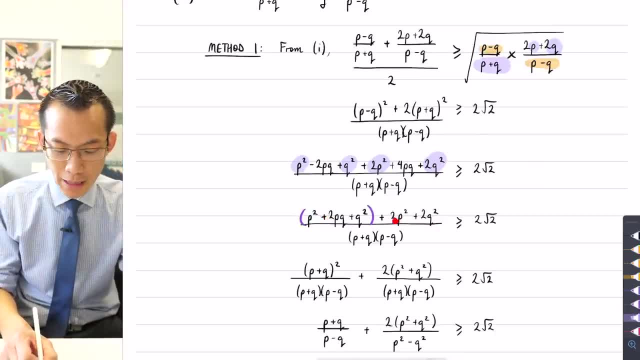 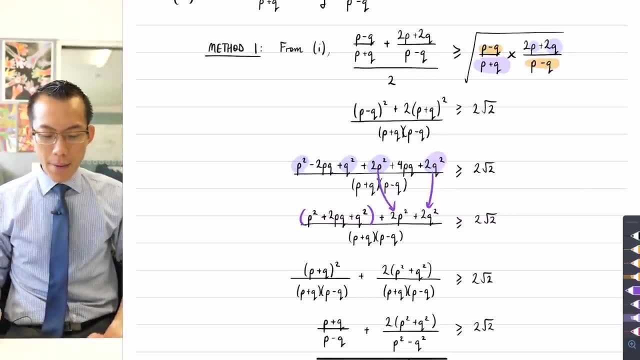 so that's how i need to do that. um, i left the t, the two p squared plus two q squared over here, so you can see that that came from here and here and then you can see from there. it's relatively straightforward. you get that perfect square factorized up here on the top. 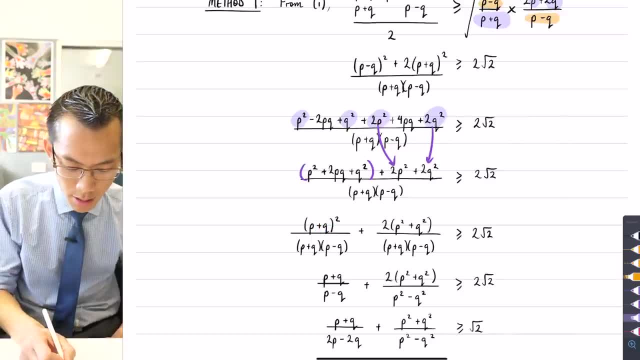 and it's going to- uh, it's going to cancel shortly, because you can see that p plus q and that p plus q they cancel. and then over here on the right hand side i want that p squared plus q squared, because if you have a look back at the result here, 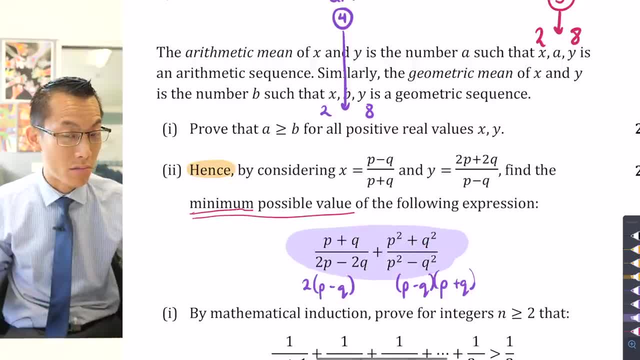 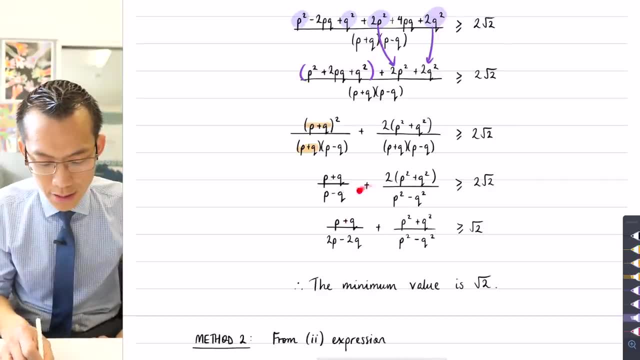 look, that's what appears right here: p squared plus q squared. i want, i want those, so that's why i didn't completely collect those like terms. you can then see, in order to go from this line to the line that i want, i had to divide back through by two, so in some senses i didn't need to multiply. 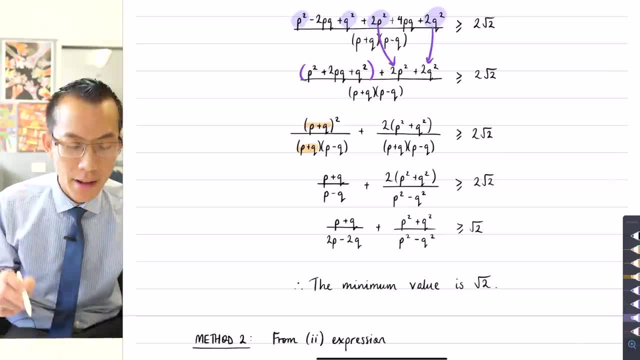 through by two um to do this simplification, but it made it tons easier for me because then i didn't have to write these two big fractions on another big fraction. now, because this is the expression i was trying to work with- i wanted to find the minimum value of this: my inequality. 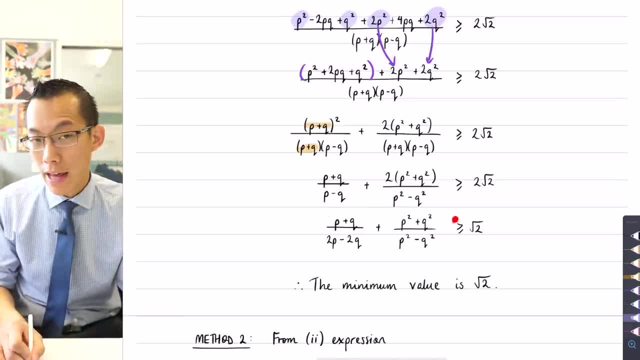 tells me that this whole expression here has to be greater than or equal to root two. greater than or equal to root two. what that means is root two is the lowest it can possibly go. in other words, the minimum possible value for this big, long expression is root two. so there you go. i've now evaluated it successfully. 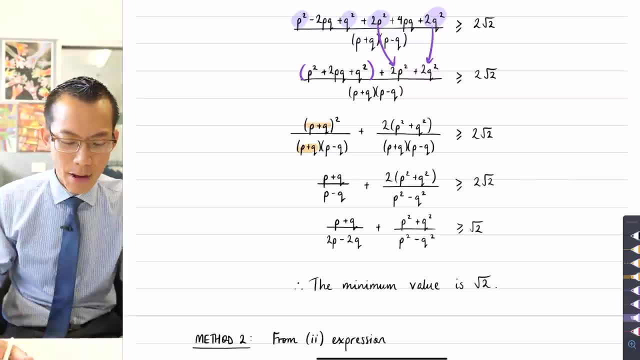 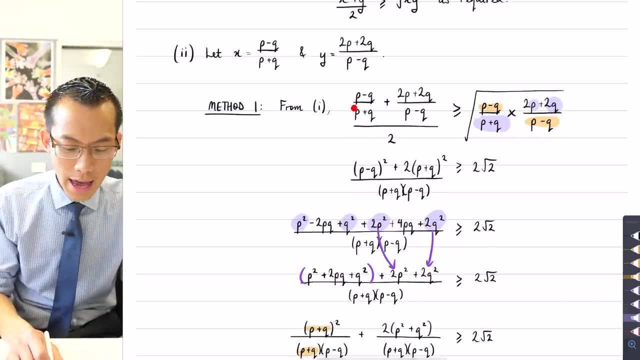 we'll show you just very quickly. even though materially it is the same. this is not the only way you can set out your solution. method one. what i did was i started with part one. i started with my am gm inequality: x plus y over two is greater than or equal to the square root of x times y. that's where i began.